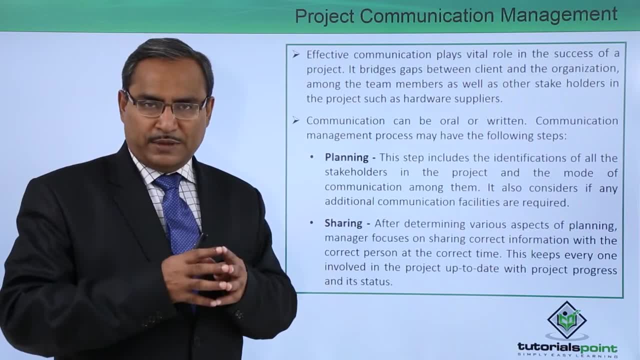 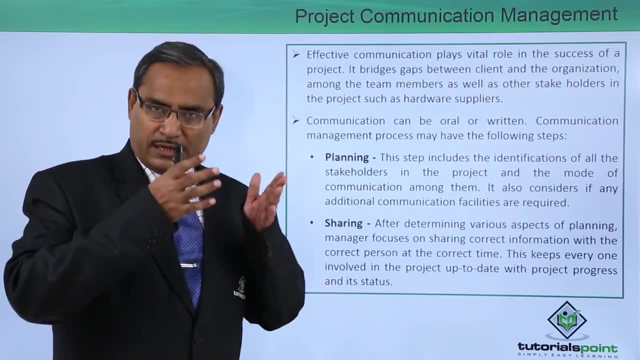 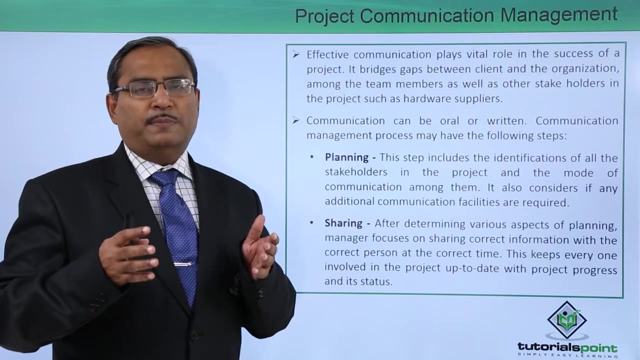 gathering should be done without any communication gap. There might be some communication gap while gathering the resource requirements. So in that case, what will happen? after we are going through the development process, after proceeding to a certain limit, We are finding that we recommend whatever we are. 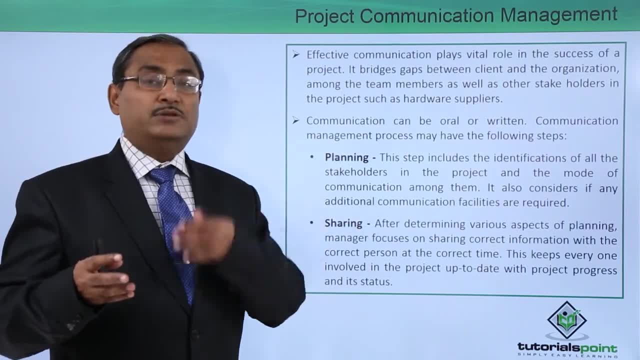 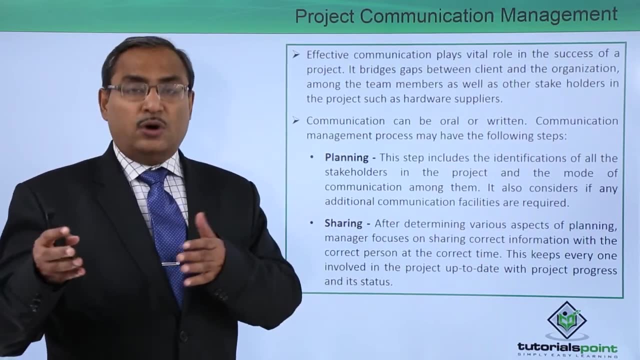 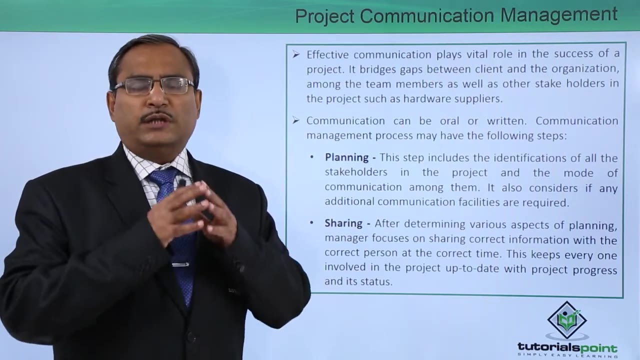 going to make. After proceeding to a certain limit, we are finding that the requirement, whatever we are implemented, that was not communicated earlier due to some communication gap: the communication gap between the team members, the communication gap with the other persons, that is, the hardware suppliers. so these are the communications should be done in a very systematic way. so there should. 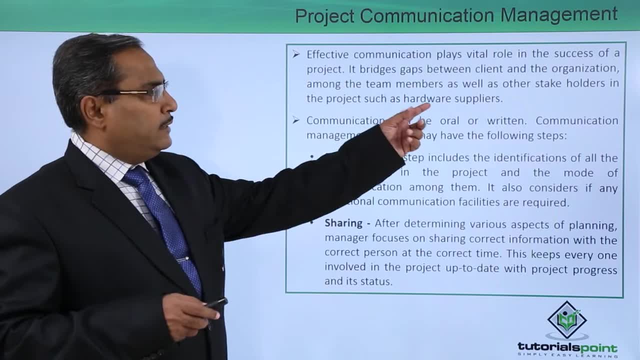 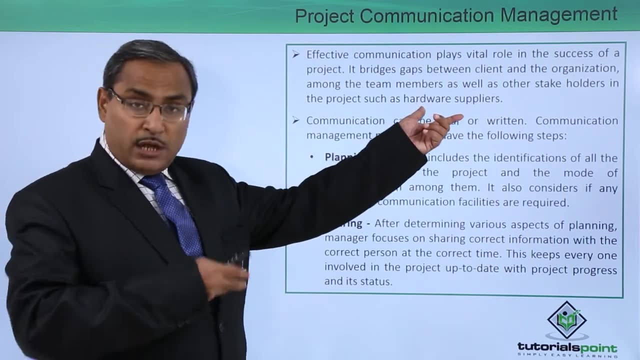 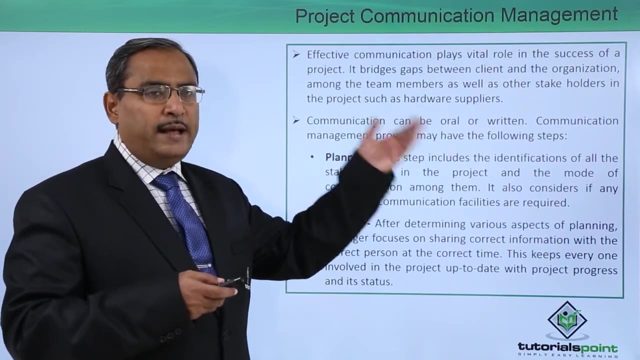 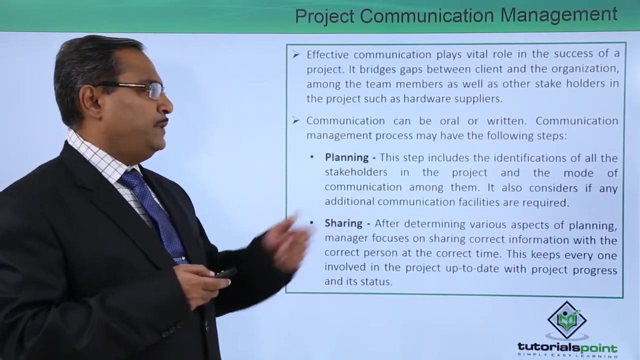 not be any miscommunication. and we know that we are having this respective stakeholders also who are getting positively or negatively affected by the execution of the project. so in between the stakeholders the respective communication gap should be none and there should not be any miscommunication, and communication can be oral or written. so communication management process. 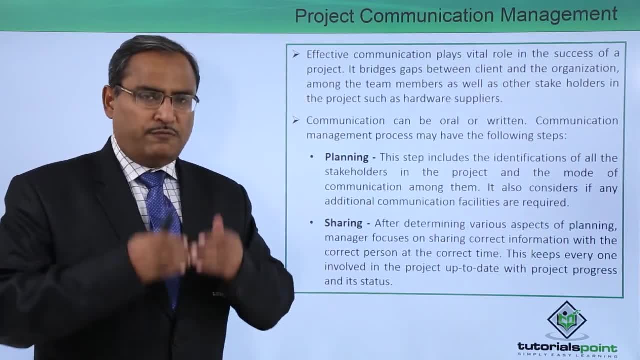 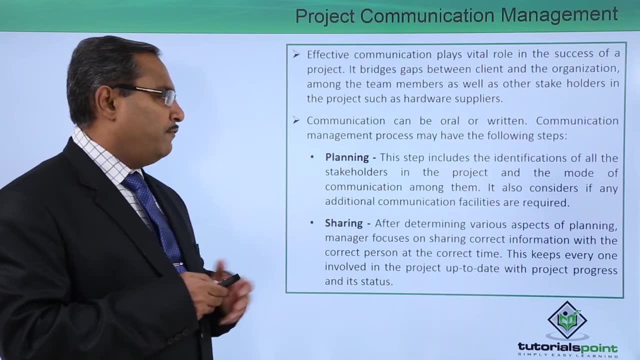 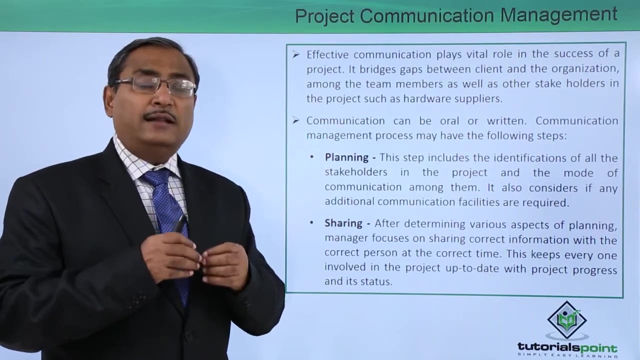 may have the following steps. so let us go through the steps for the better understanding. so at first we are going for this planning. so this step includes the identification of all the stakeholders in the project. so at first we should identify all the stakeholders in the project and the respective mode of communication and the respective mode of. 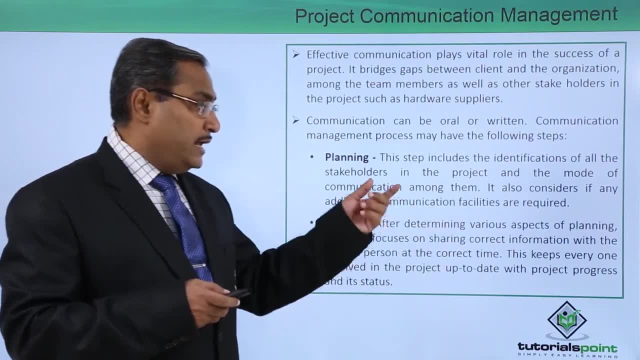 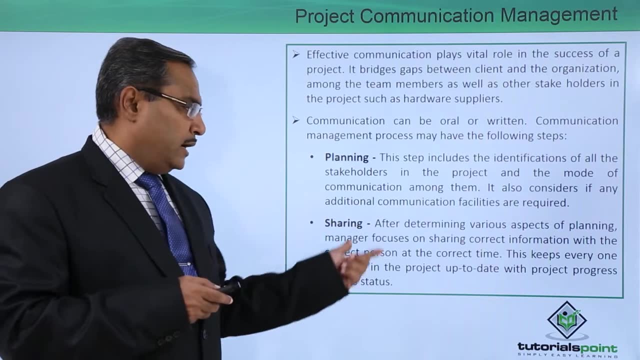 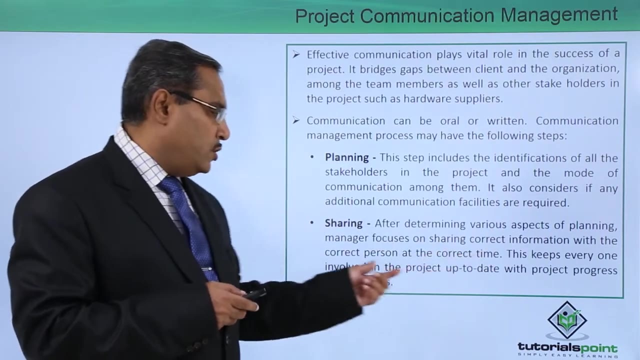 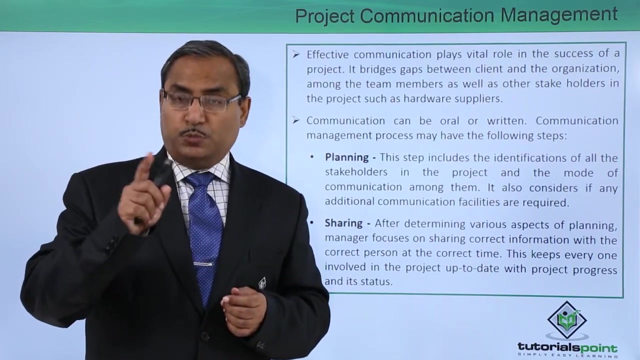 communication. among them, it also considers if any additional communication facilities are required. next one is the sharing. after determining various aspects of planning, manager focuses on sharing correct information with the correct person at the correct time, so correct information should be propagated, should be shared with the correct person at the correct time, so the correct information. 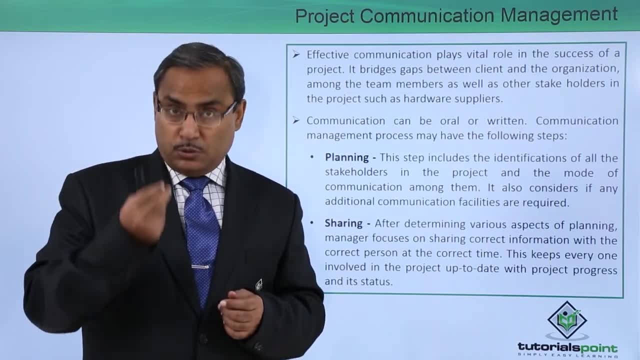 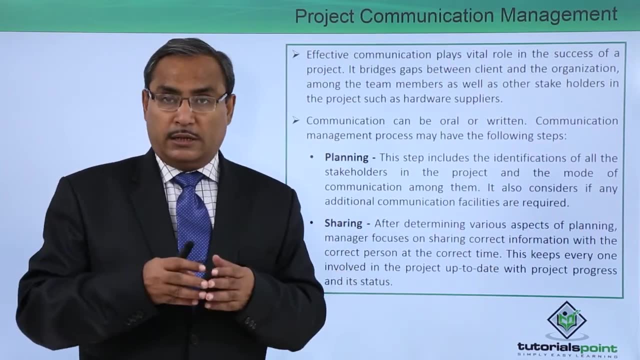 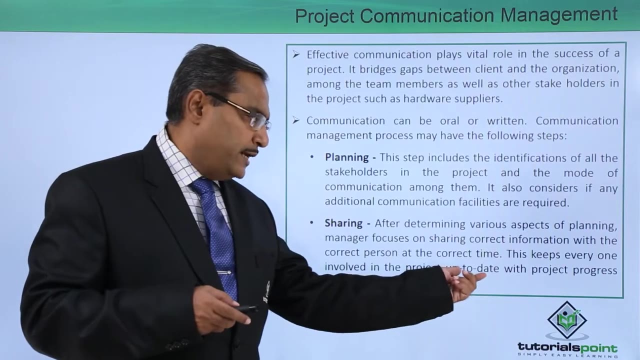 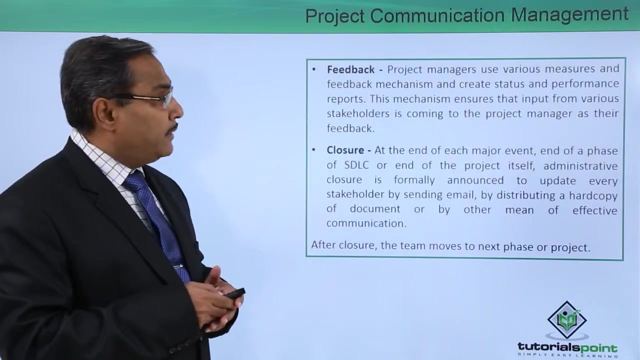 should be shared with the correct person who is actually responsible to, to have that respective communication at the correct time. so the communication should not be delayed, otherwise some different anomalies may come into the system. this keeps everyone involved in the project up to date and with project progress and its respective status. next one: we are considering this feedback. 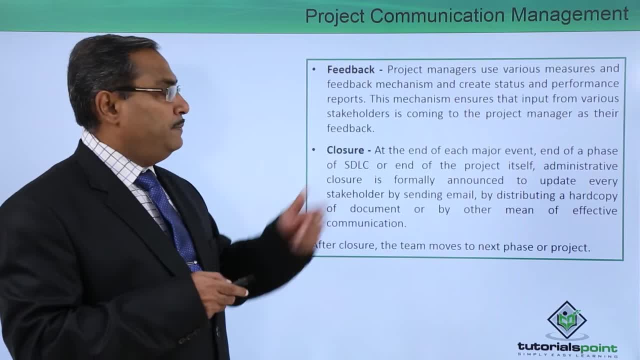 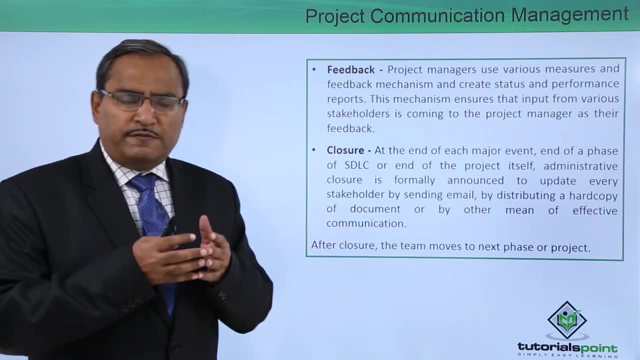 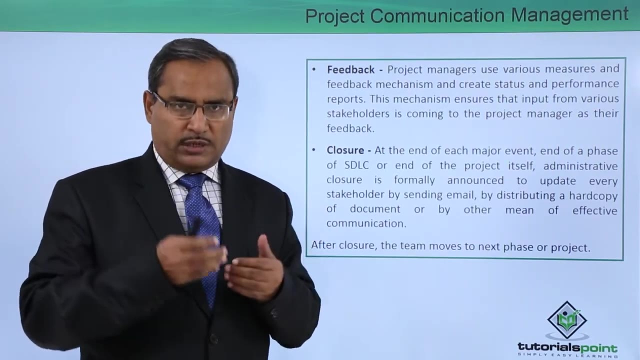 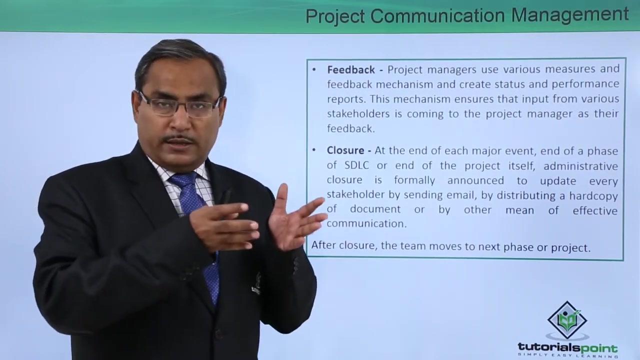 so project managers use various measures and feedback mechanism to create status and performance reports. so let us suppose just consider different tasks are there? so whenever we are doing the weekly study on those tasks, or say day-to-day study on those tasks, so these tasks can have, say, three different kinds of status. so one is the in operation or ongoing, another one is 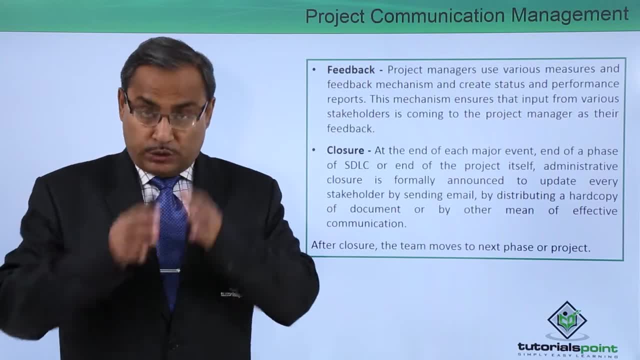 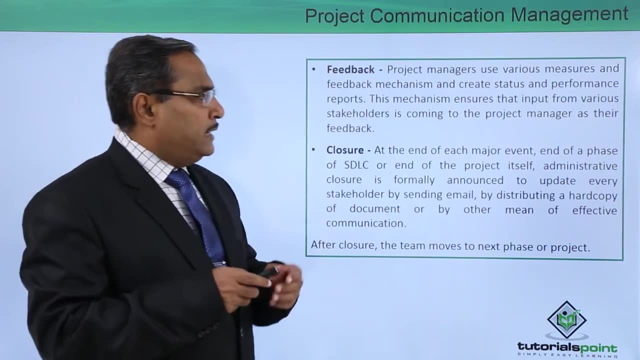 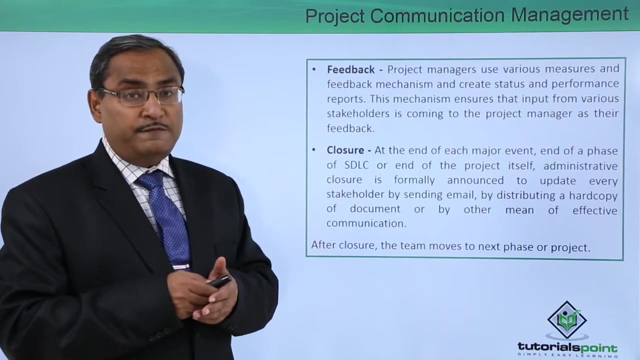 a pending and the one is a finished, so this sort of status reports must be communicated with the respective person's at the right time. this mechanism ensures that input from various stakeholders is coming to the project manager as their feedback. so the project manager should have the access, or should. 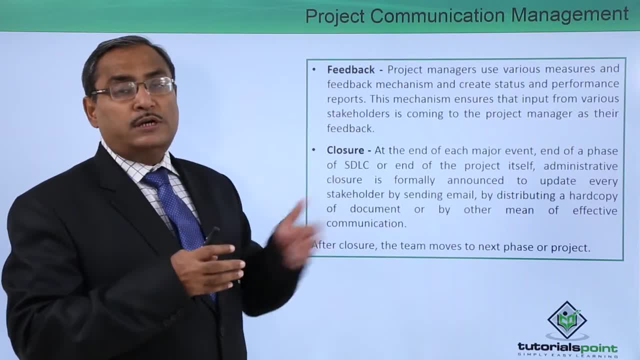 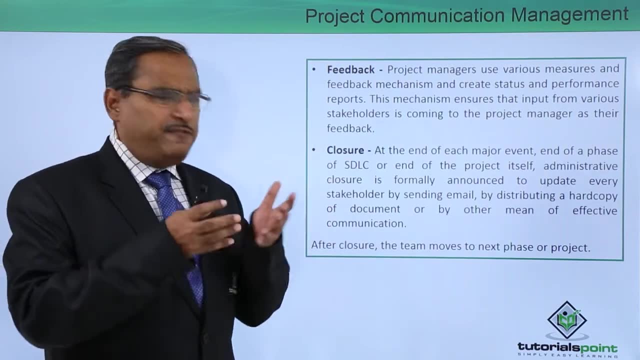 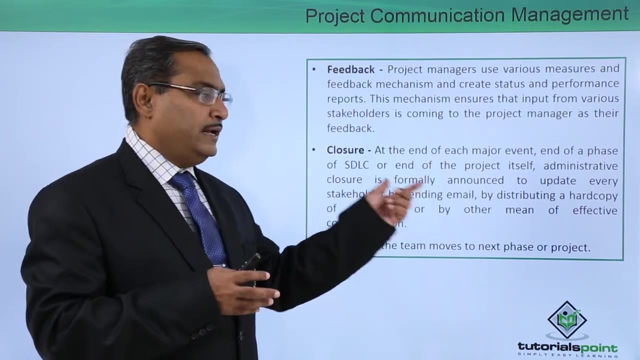 have be getting all this respective stakeholders feedbacks. so next one is the closer at the end of each major event or end of some phase of the respective sdlc or end of the project itself. administrative closer is formally announced to update every stakeholder by sending email. 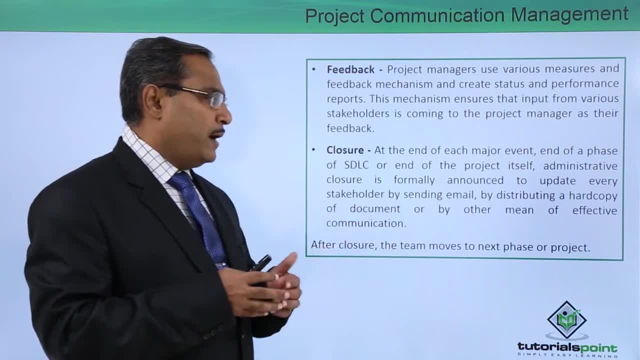 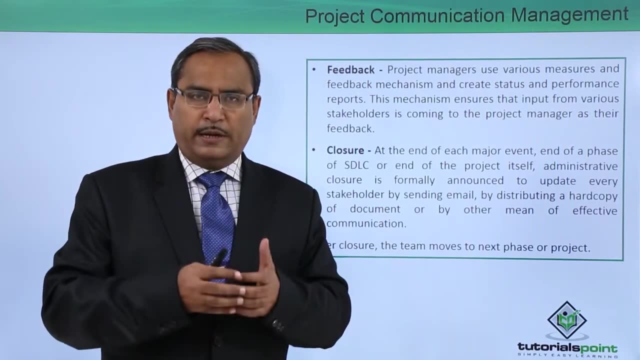 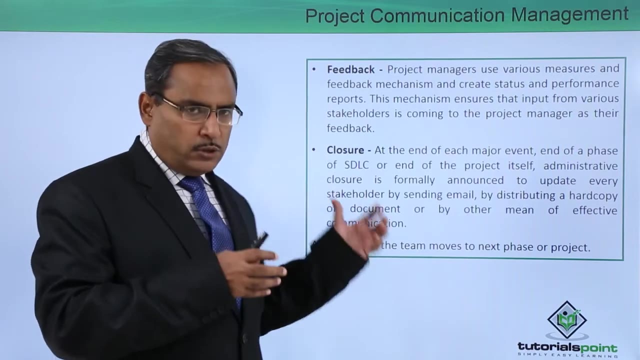 by distributing a hard copy of the document or by other means of effective communication. whenever a project will get will get the closer, or whenever a particular phase or the major activity is going to get a closer, then obviously the respective stakeholders should get that information either through mail or using some special 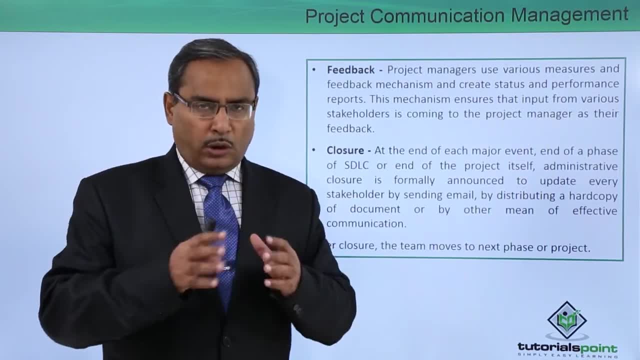 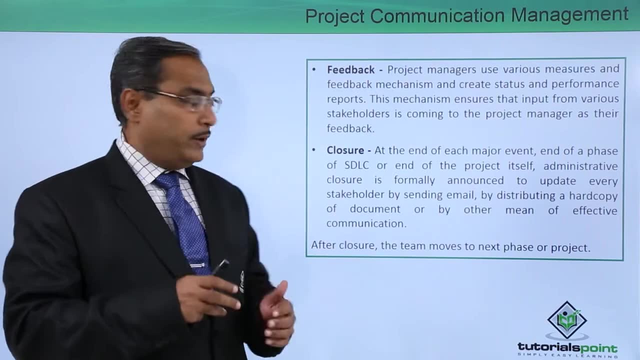 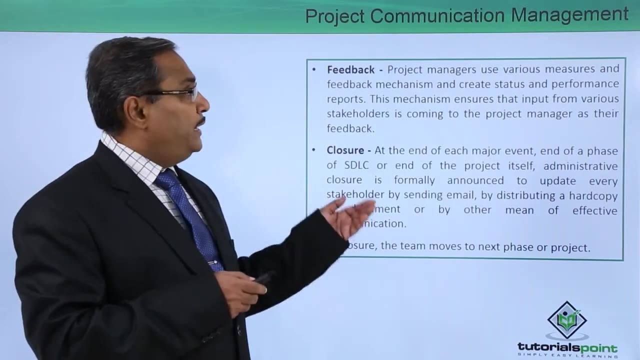 kind of formatted documentation. so somehow all the stakeholders and the related personnel should get those information at the right time in a properly documented way. so after closer the team moves to the next phase or the next new project. so in this way we have discussed that in our project. 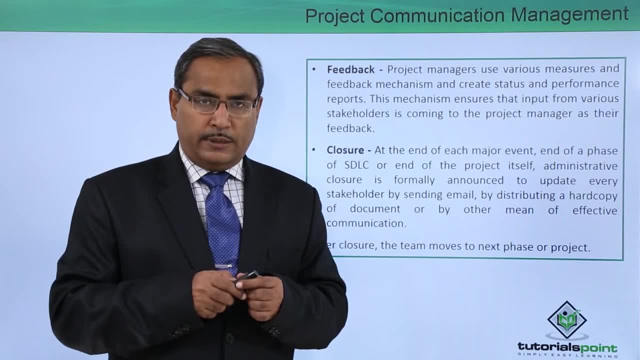 how the communication management can be done. thanks for watching this video tutorialscom- simply easy learning.